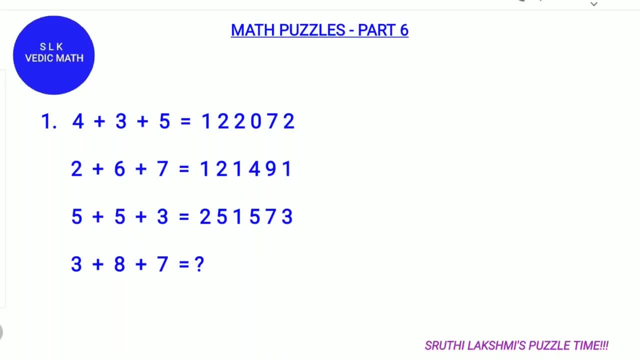 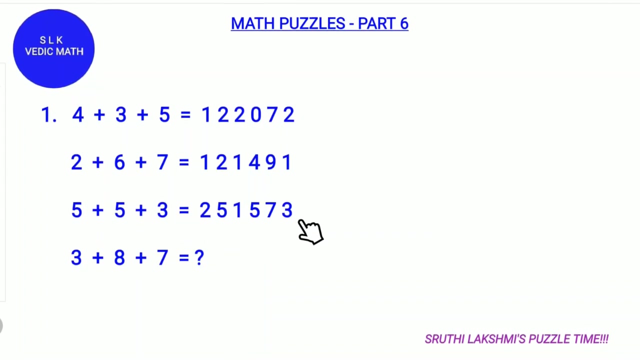 Hi, welcome to Shruti Lakshmi's virtual classroom. Today we are going to see few math puzzles. Puzzle number 1.. 4 plus 3 plus 5 is 122072.. 2 plus 6 plus 7 is 121491.. 5 plus 5 plus 3 is 251573.. 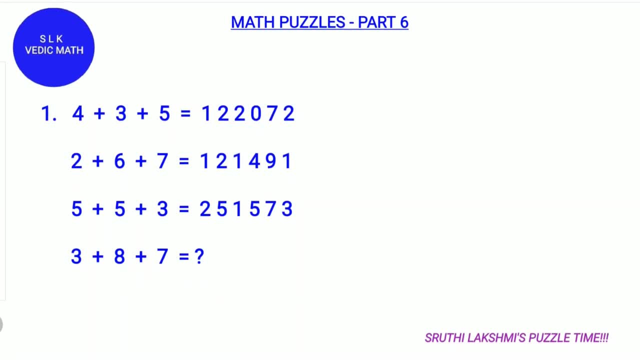 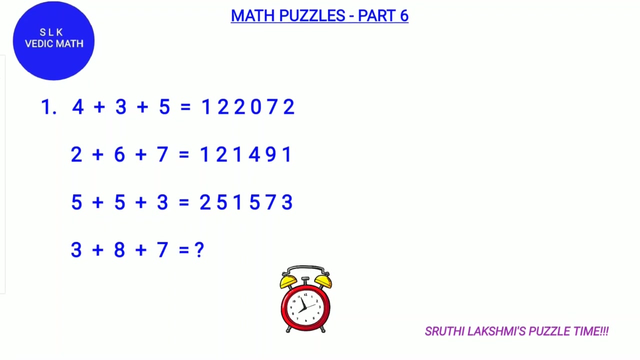 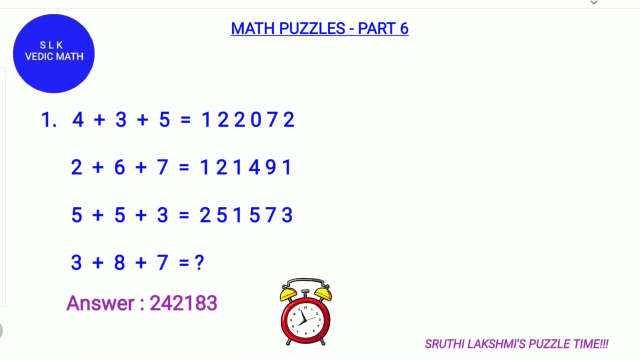 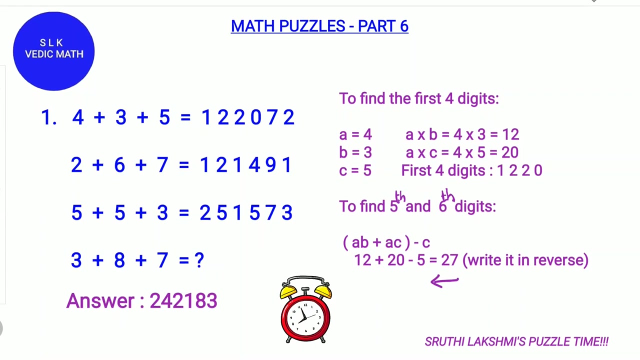 So what is 3 plus 8 plus 7?? You will have 20 seconds to solve this problem, Starting now Time's up. The answer is 242183.. For 4 plus 3 plus 5, to find the 4 first digits, we do 4 times 3,, which is 12, and 4 times 5,, which is 20.. 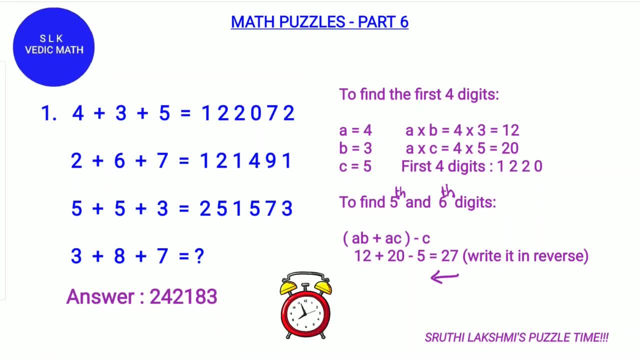 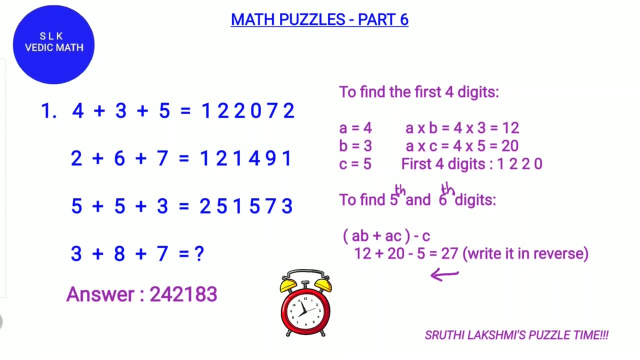 Next, to find the 5th and 6th digits, we do 4 times 3,, which is 12., And 4 times 5,, which is 20.. We add 12 plus 20,, which is 32, and we subtract the last digit of 5.. 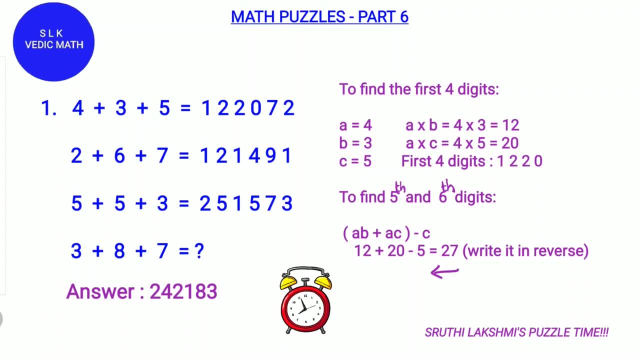 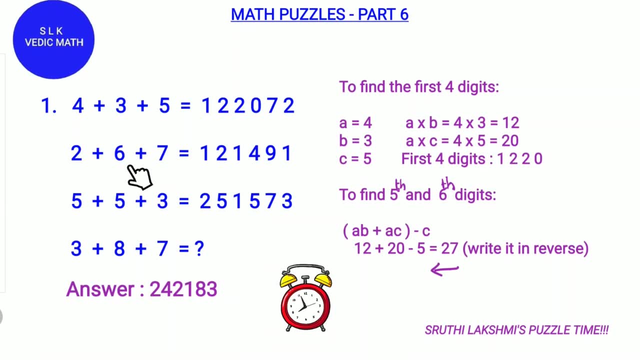 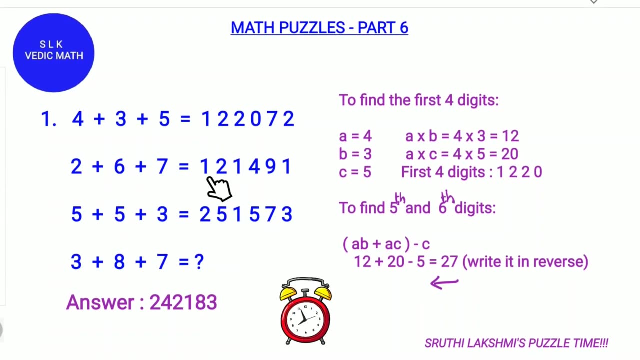 So 32 minus 5 is 27.. We write 27 in reverse, which is 72.. For 2 plus 6 plus 7, we do 2 times 6,, which is 12,, and 2 times 7,, which is 14.. 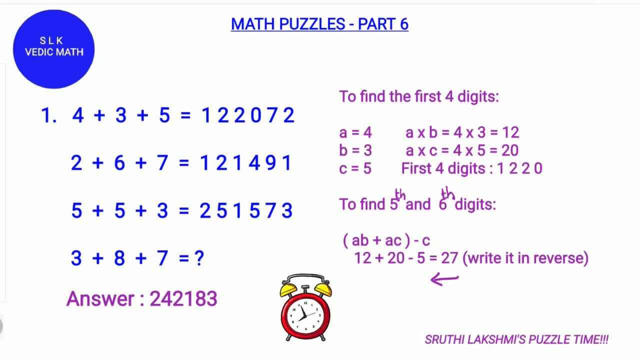 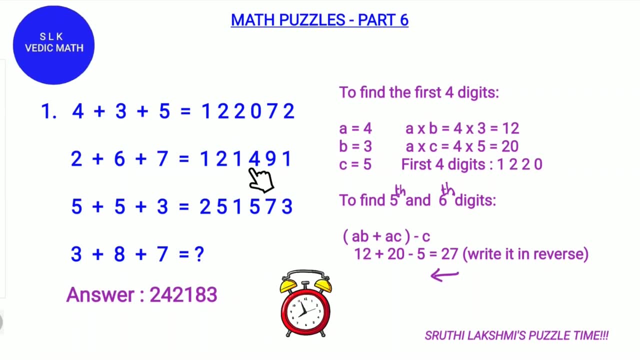 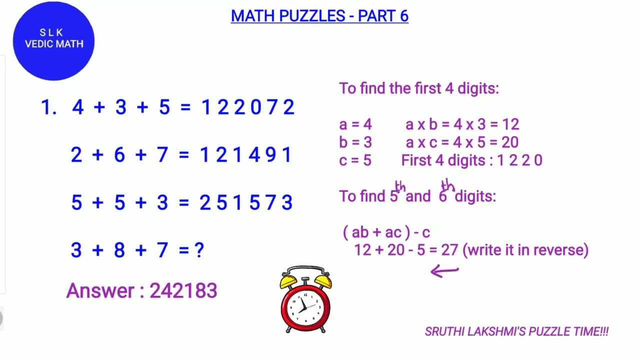 To find the 5th and 6th digits, we do 2 times 6,, which is 12,, plus 2 times 7,, which is 14.. So 12 plus 14 is 26.. And 26 minus the last digit, 7, is 19.. We write 19 in reverse, which is 91. 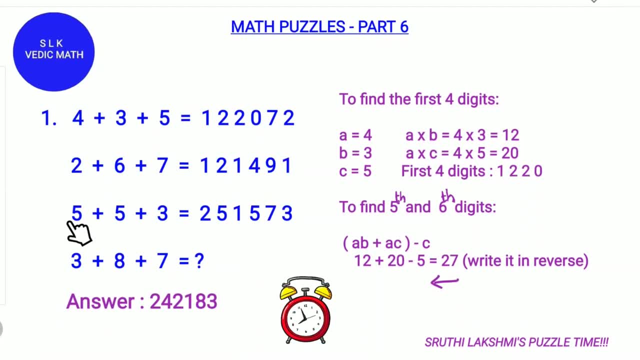 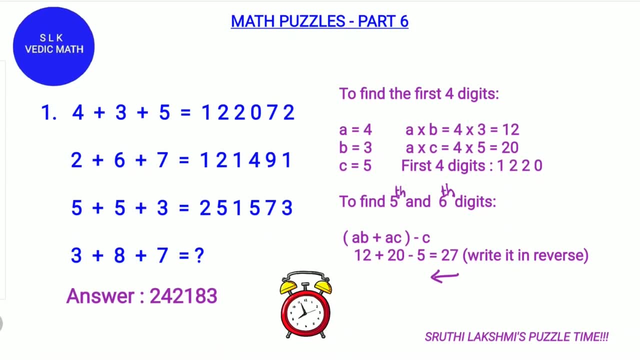 For 5 plus 5 plus 3, we do 5 times 5,, which is 25.. 5 times 3,, which is 15.. We add 25 plus 15,, which is 40, and we subtract 3 from 40,, which is 37.. 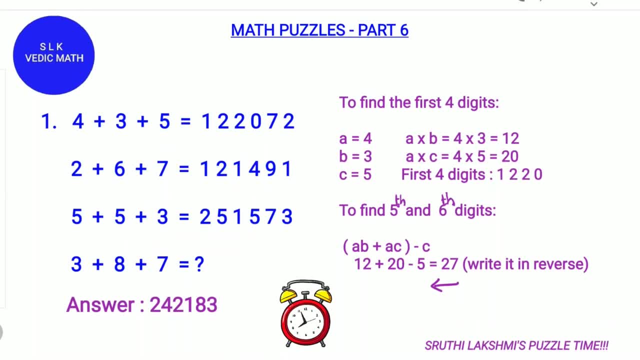 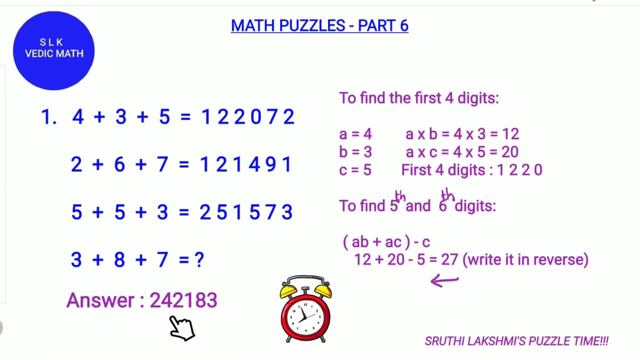 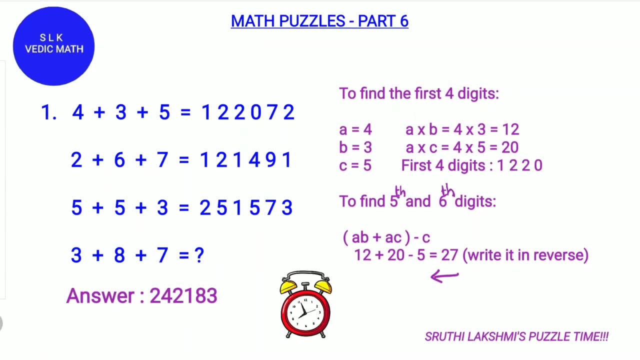 And we write 37 in reverse, which is 73.. For 3 plus 8 plus 7,, we do 3 times 8,, which is 24,, and 3 times 7,, which is 21.. Next we add 24 plus 21,, which is 45,, and we subtract the last digits. 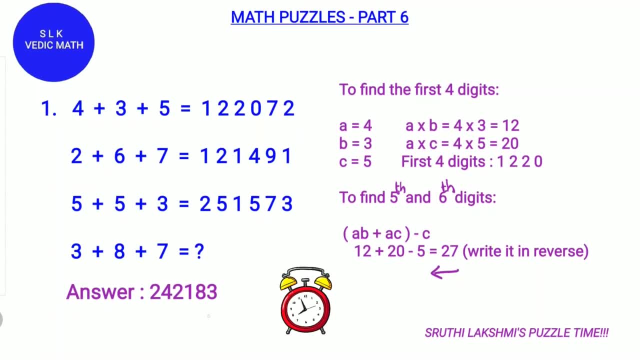 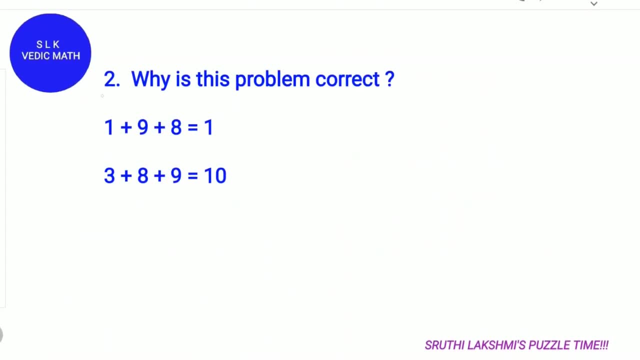 7 from 45.. 45 minus 7 is 38. We write 38 in reverse, which is 83.. Puzzle number 2.. Why is this problem correct? 1 plus 9 plus 8 is 1.. 3 plus 8 plus 9 is 10.. 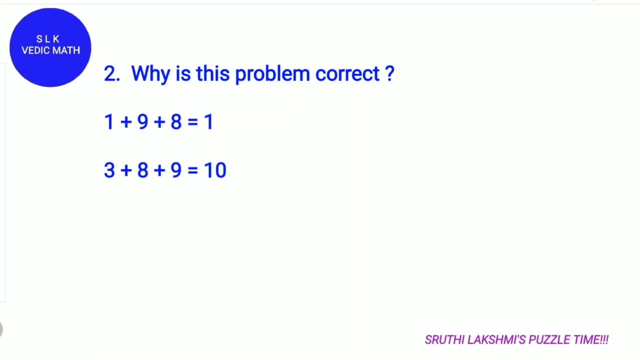 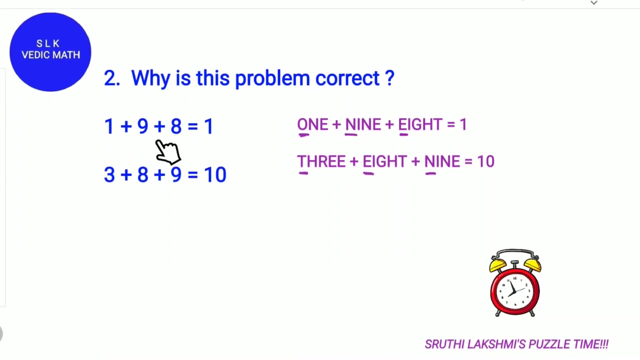 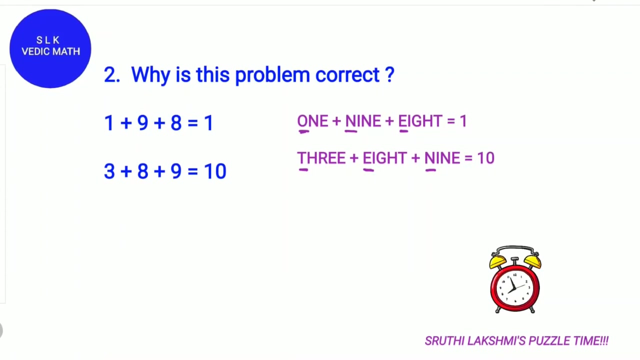 You will have 20 seconds to solve this problem. Starting now, Time's up. First, for 1 plus 9 plus 8,, we write 1 in word form. We write 1,, 9, and 8 in word form. 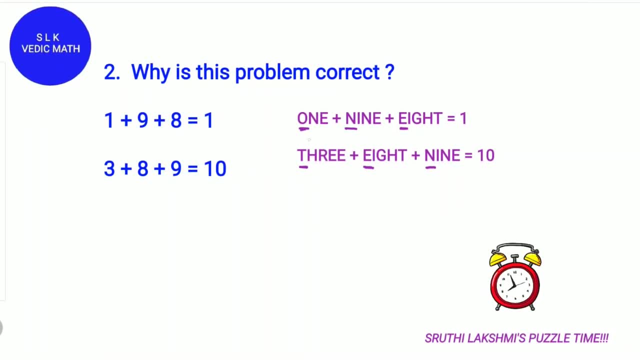 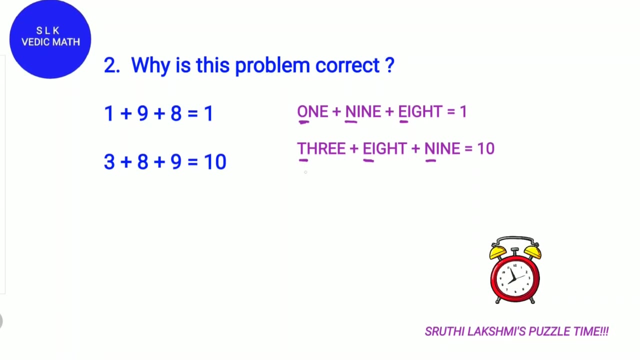 We take the first letters from 1,, 9, and 8,. so O N E is 1. For 3 plus 8 plus 9, we do. we write 3,, 8, and 9 in word form and we take the first letters T, E and N. 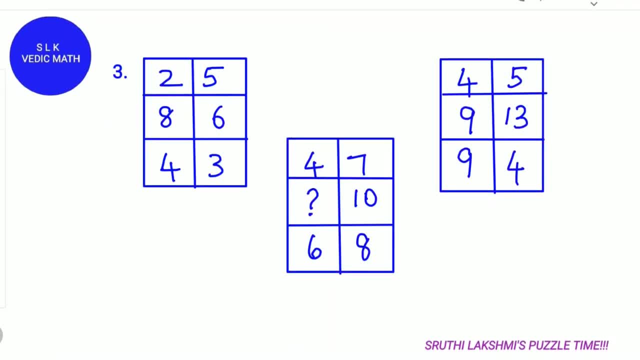 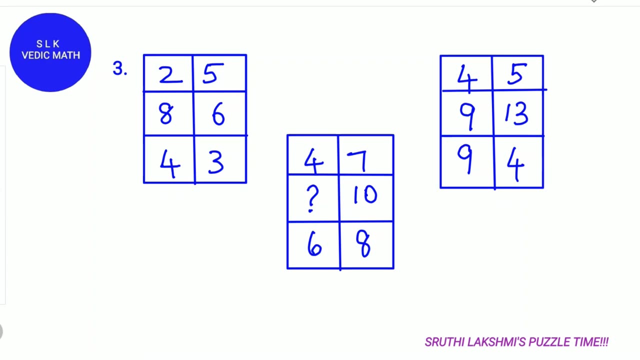 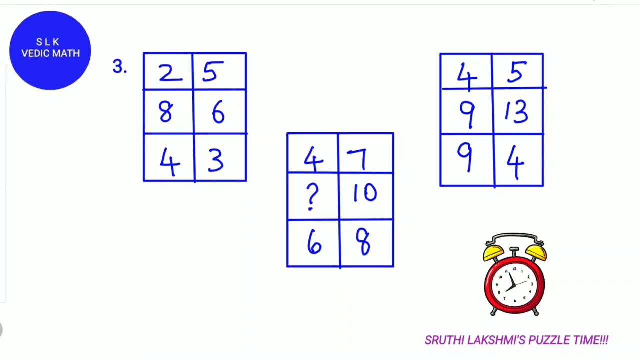 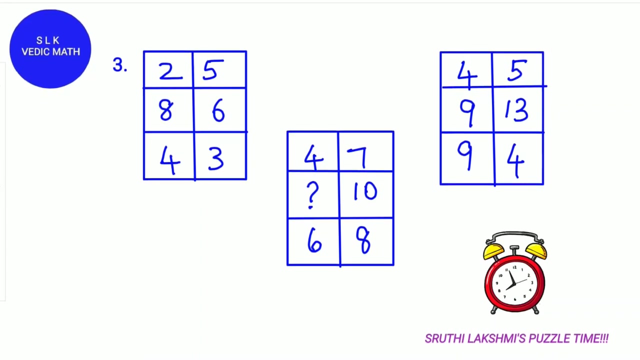